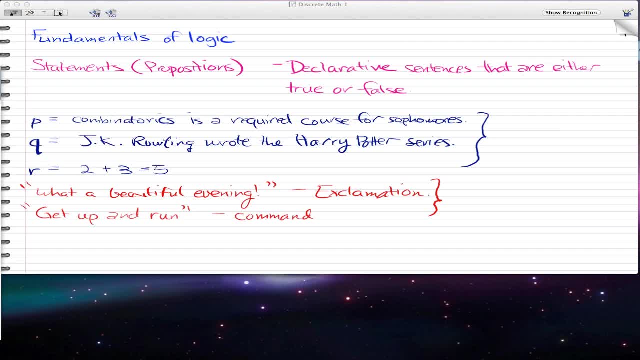 okay, so we're on fundamentals of logic and what i want to say is: you guys better do well in fundamentals of logic, because in discrete mathematics, well in like the first, first couple of chapters in discrete mathematics or your first term in discrete mathematics- one fundamentals of logic is going to save your ass if you're doing poorly in the whole entire course. so, without 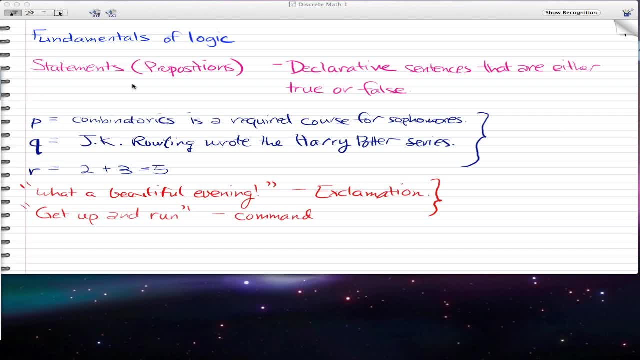 further ado, let's get on with it. so the first thing you got to do is we got to know some definitions. like like any of like learning anything else. you got to know some definitions. so first we got to learn what a statement or proposition is now. propositions or statements. 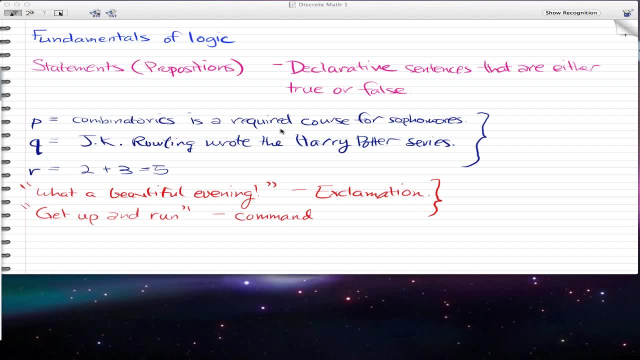 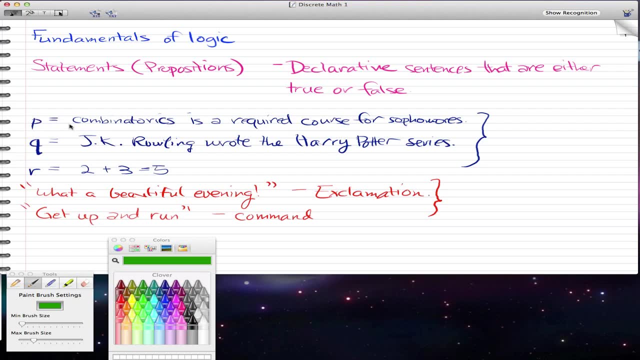 are pretty much the declarative sentences that are either true or false. so let's look at these statements that we have here. that i have in blue. commonatorics or pp is uh, combinatorics is a required course for sophomores key. you, jk rowling, wrote the harry potter series and r 2 plus 3 equals 5.. now what we call these? 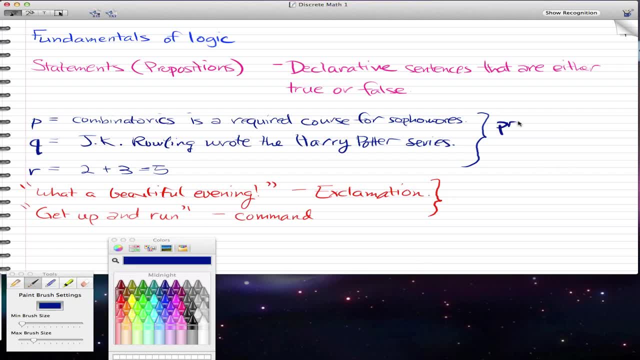 is we call them primitive statements. so we call them primitive statements for a reason: primitive statements. and you can see that i've actually changed my app because cario fucking fucking shat on me and it got destroyed. but but we're going to talk about primitive statements. now let's talk about pq and r. 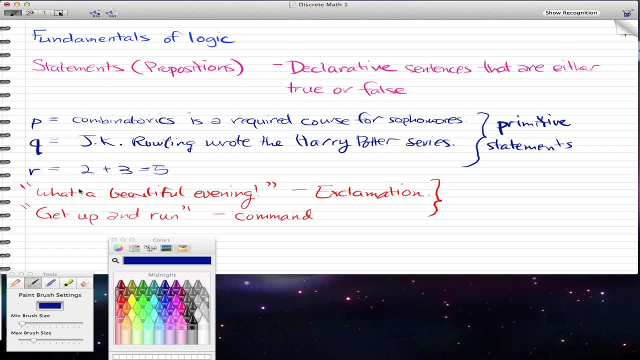 because pq and r are called primitive statements. why are they called that? because they are fact. that that is. they are either true or they're false. they're declarative statements or declarative sentences that can be said as true or false. now, how about these two sentences? what a beautiful. 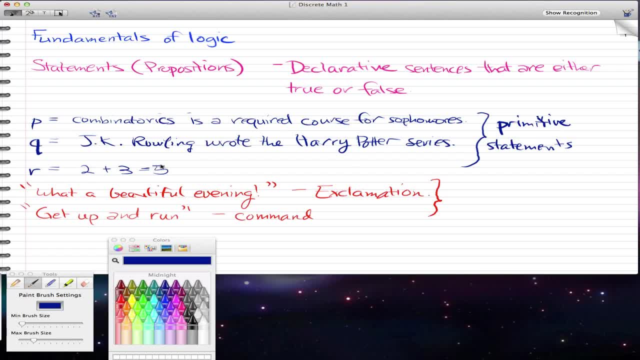 evening there's an exclamation: and get up and run. that's a command. what do you think are these primitive statements? well, they're not primitive statements. the reason is because they vary. what a beautiful evening. well, evenings can be rainy, sunny, or cold or hot, so you can't that. 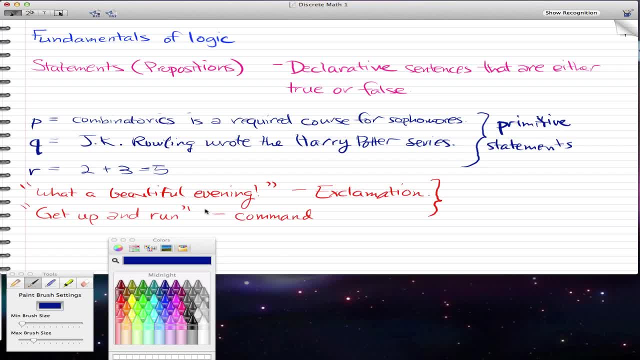 you can't really say if it's true or false that. so that's really not a primitive statement. get up and run that command. that can happen at any time. it can happen. uh, it can happen when you wake up, or it can happen while you're sitting on a chair, so that varies as well. so we do not regard. 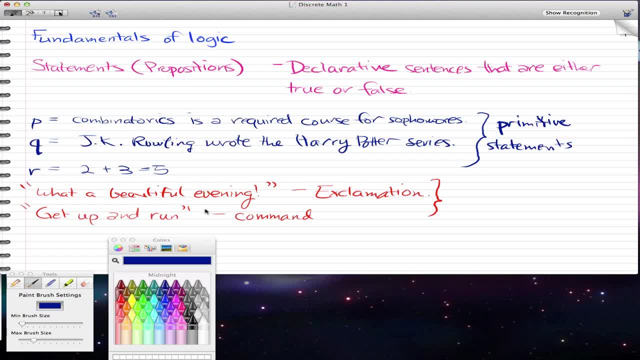 sentences such as exclamation or commands, as statements, because they vary. they vary, they don't have a truth value, so they can't really be said true or false at any time, but for primitive statements, they primitive statements, can be said, can be answered as true or false at 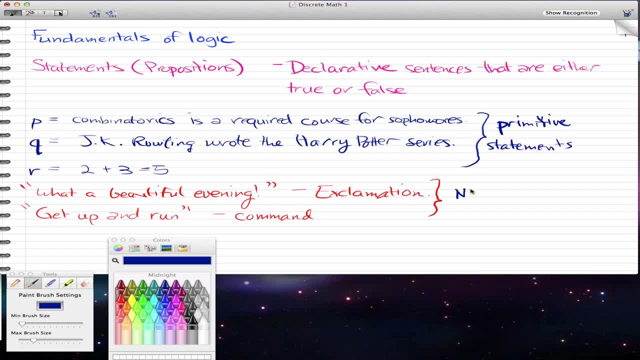 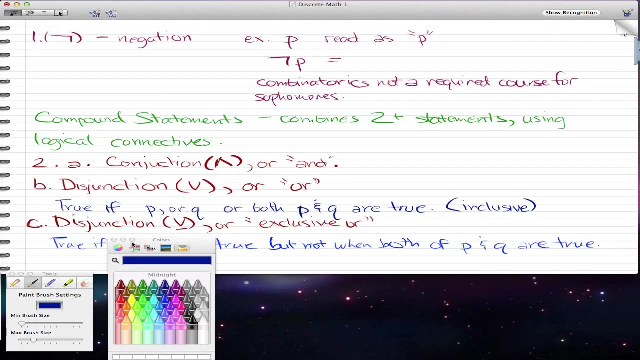 any time, so that's why they're called primitive statements. so these ones are not, uh, not primitive statements. so now that we've gone through that, let's go ahead and continue. so what we have now is a couple of rules that you gotta learn before doing anything else in fundamentals of logic. 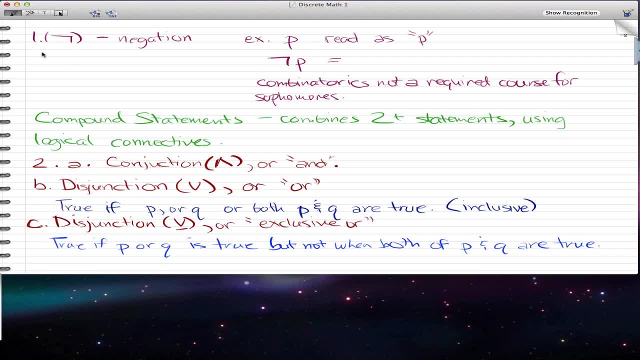 and the first thing you gotta learn is negation. and this, the symbol for negation, is kind of like a gun. so if you see a gun like, like symbol, then that's negation. so let's, for example, let's say that p is read as p, then what would we read? uh, shotgun, ps. well, what we'll read it as is that: 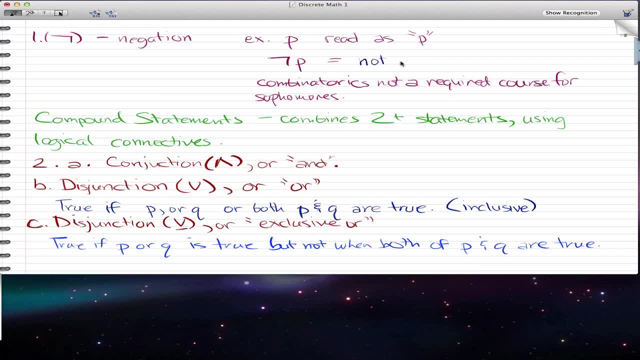 we'll read it as uh, not p, not p. so that is what the negation means. if we have a p, then we just negate it. so if i said, uh, that you have to take this math, math course, then putting that shotgun in front of that statement would be: you don't have to take that math course. so that's the idea behind negation. 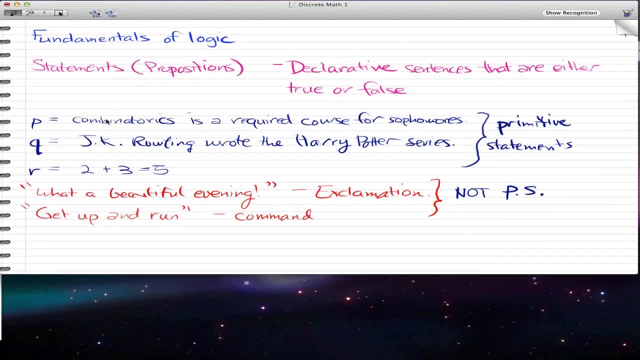 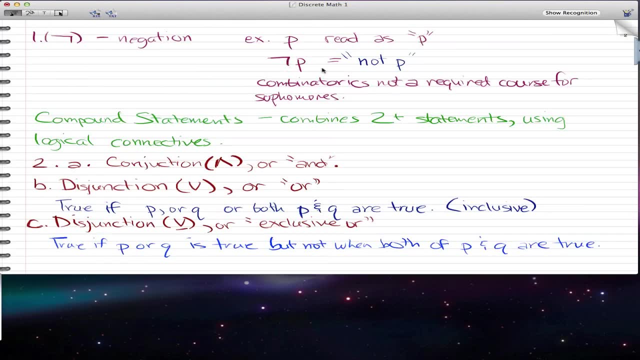 so if, for example, our p in the last statement was: combinatorics is a required course for sophomores, if we put a shotgun in front of the p, then it'll read: commentaries is not a required course for sophomores, and that's the. that's the basis behind uh, behind negation. now, compound statements are. 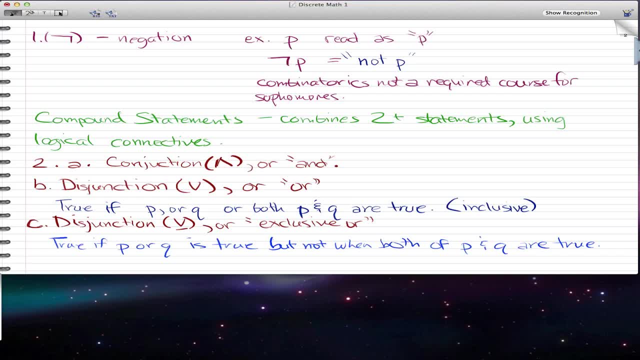 a little different. they're not as simple as negation, but they're. they're still pretty simple. so the first one i want to go through is conjunction, and this is: this is the symbol for conjunction, and it's written as an upward carrot and it's read as: and so if we put p, 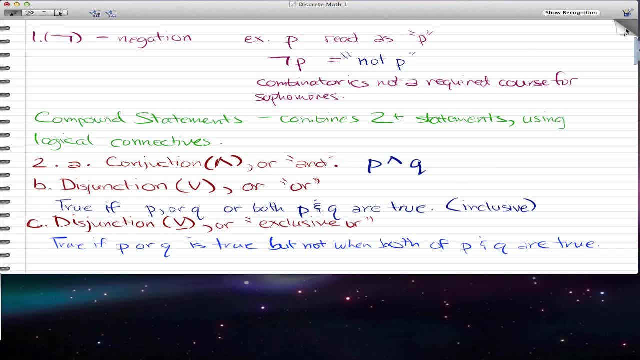 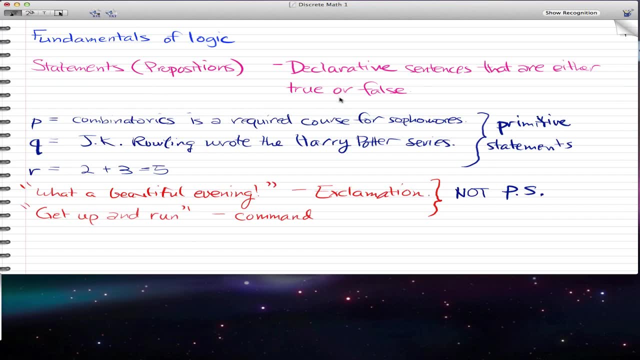 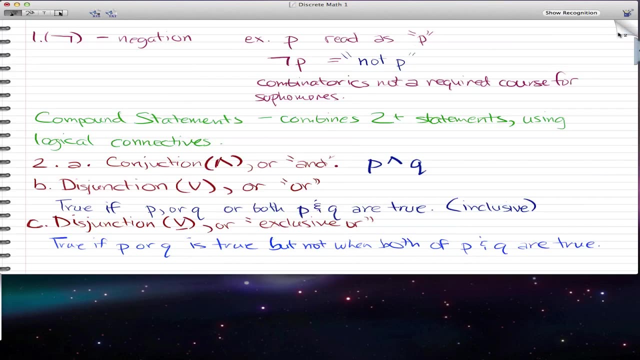 carrot q and that is read as p and q. and referring back to the statements that we had p and q, it will be read as: commentorics is a required course for sophomores and jk rowling wrote the harry potter series, so that's how we read those statements, with the conjunction and: 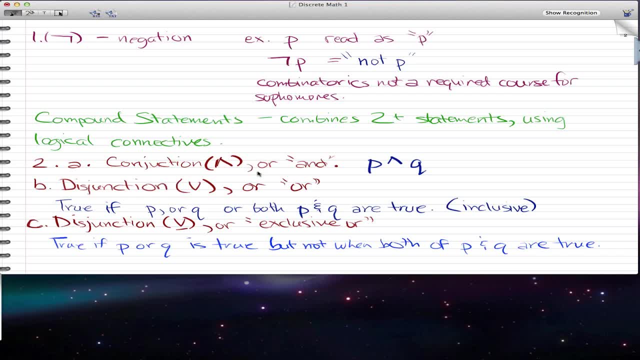 and now b disjunction. this is an inclusive disjunction because there's two. there are two kinds of disjunctions. as you can see. b and c are both disjunctions, but for b we just have, uh, an upside down caret symbol and for c we have upside down caret symbol and a bar under it. 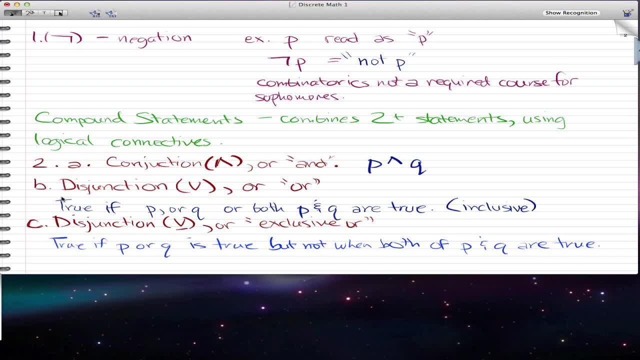 so b is read as or, and it's true if p or q or both p and q are true. so that's what we mean by inclusive. so this could be right. this could be written as p under up, upside down carrot symbol and q or that is equal to p or q. so this is this statement is true when we say that. commentorics: 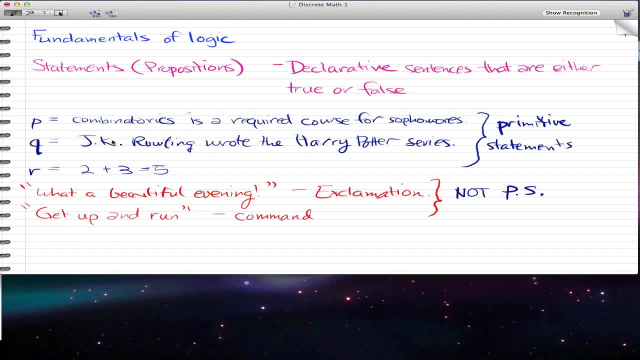 is a required course for sophomore, or jk rowling wrote the harry potter series, or common torch is a required course for sophomores, and JK Rowling wrote the Harry Potter series. So if P or Q is true, or P and Q is true, then that statement is true. 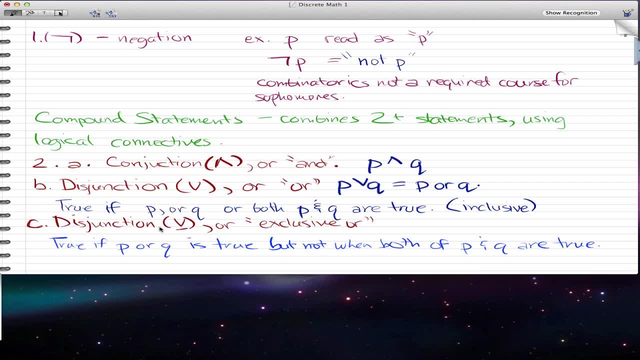 Now let's go back. Disjunction with the exclusive disjunction is the opposite. It's true only if P or Q is true, but not when both P and Q are true. So in this case, we will consider it true when combinatorics are required for sophomores. 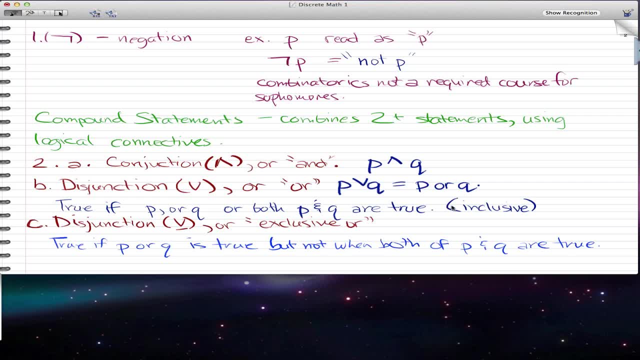 or when JK Rowling wrote the Harry Potter series. But if there is a statement that says combinatorics is a required course for sophomores and JK Rowling wrote the Harry Potter series, then that is not true in this case. So it's written as P and Q. 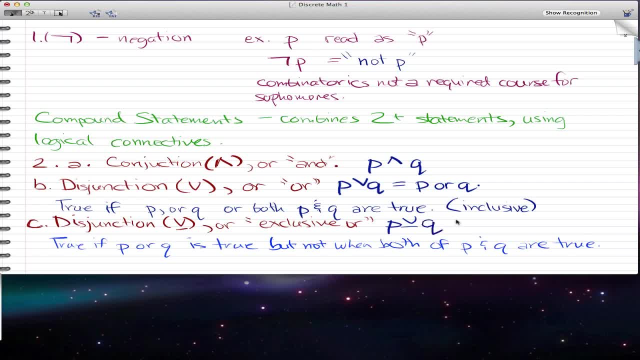 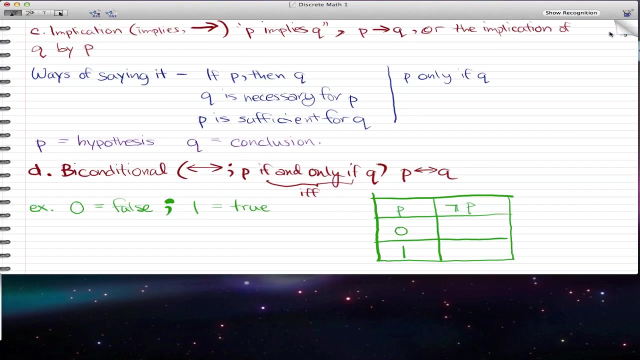 So if P or Q is true or P and Q is true, then both P and Q are true, and exclusive disjunction is true when P or Q is true, but not when both P and Q are true. So, moving on, we have implications. 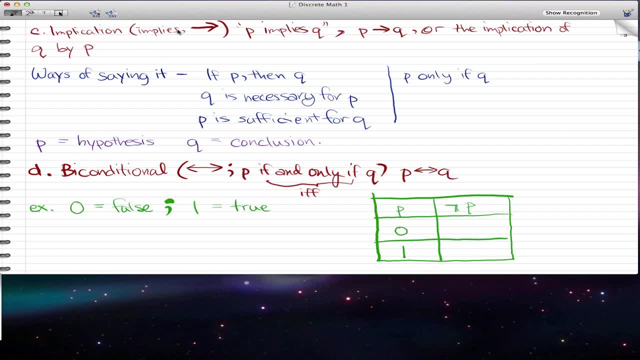 So this is symbolized by an arrow and this arrow pretty much means implies. So if we have P implies Q, that's pretty much P arrow Q or the implication of Q by P. There are different ways of saying it, Such as: if P, then Q, Q is necessary for P, P is sufficient for Q and P only if Q. 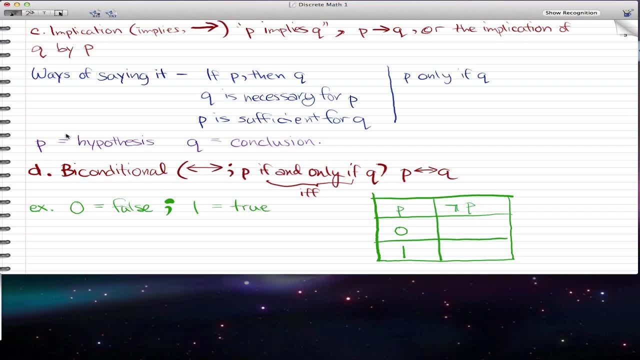 Now, P in this whole statement is the hypothesis and Q is the conclusion. And an example of this is using our combinatorics and Harry Potter example. then we could say that the statement for P implies Q is: If combinatorics is a required course for a sophomore, then JK Rowling wrote the Harry. 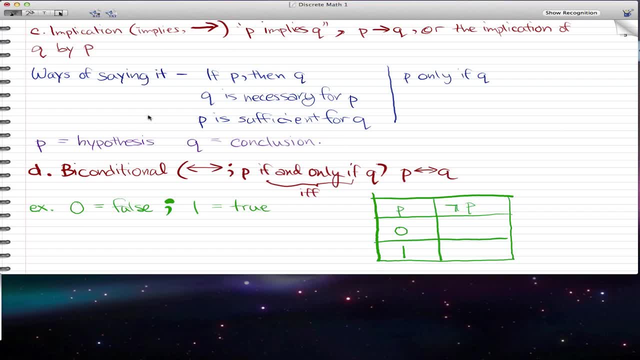 Potter series. So that's an example of how you would give the statement, for P implies Q, with P and Q representing those two statements. D is a biconditional and this is represented by an arrow with two arrowheads on both sides. 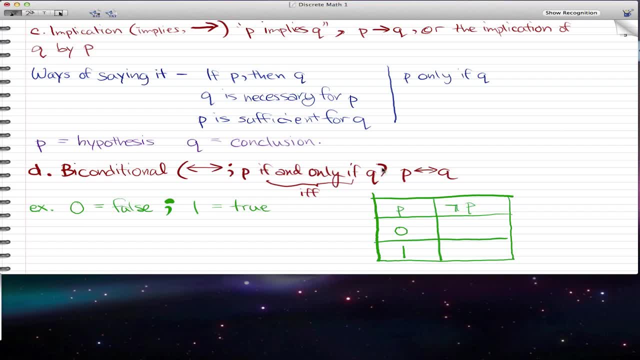 and it is P, If and only if Q. So this only happens if P. if Q happens, then P must happen. if P happens, then Q must happen. That is why we have that if and only if. So this you might have done in high school, because I think indirectly every high school.